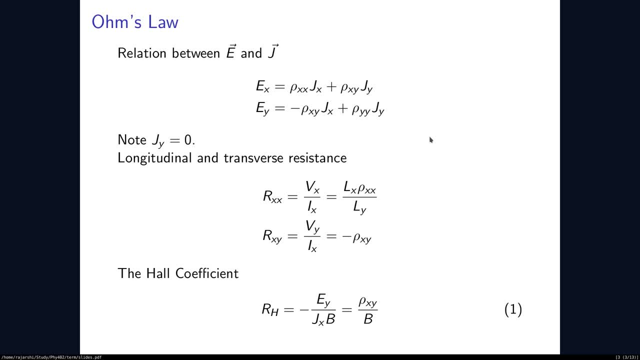 in our case the current is made to flow in the x direction, So J y is 0.. The resistance, the longitudinal resistance, R x, x is V, x by I, x, and it is related to the resistivity with some geometrical parameters. Over here it is L x and L y. L x and L y are the lengths. 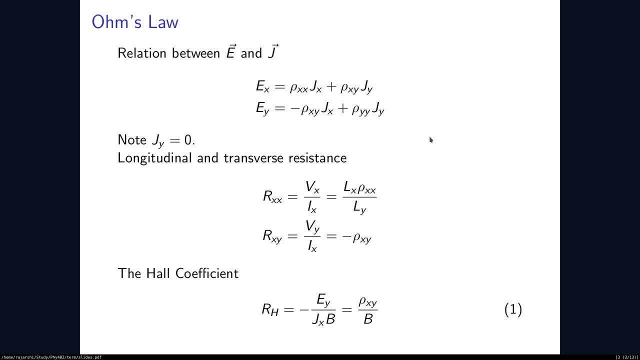 of the material in the x and the y directions. Interestingly, when we look at the transverse resistance, which is V- y by I- x, it is directly related to the resistivity x- y and it does not depend on the geometrical properties. So we can imagine that when we increase the 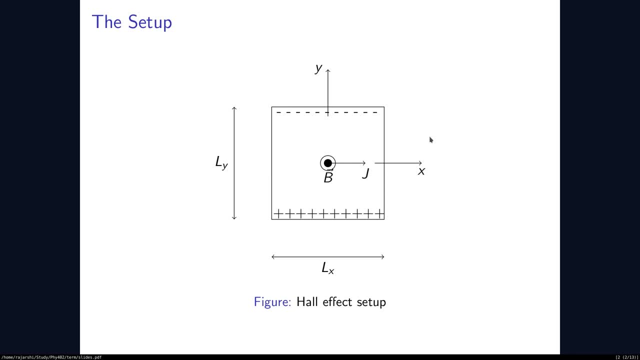 magnetic field. the charges are going to accumulate more and more because the force is larger, And because of this larger force the potential will be higher. So we can imagine that rho, x, y may be proportional to B, and this proportionality constant is called the Hall coefficient. Now 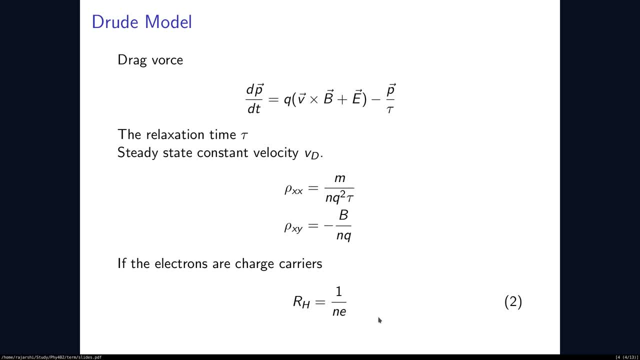 that we understand the setup. let us understand what the Drude model has to say about this. So in the Drude's model we talk about the momentum averaged over a particular time. So we talk about average momentum And the momentum is averaged over the time scale of. 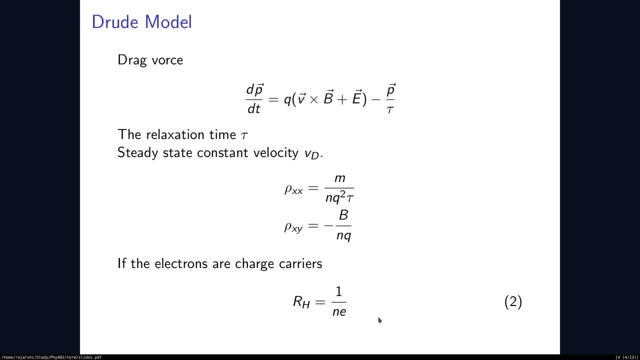 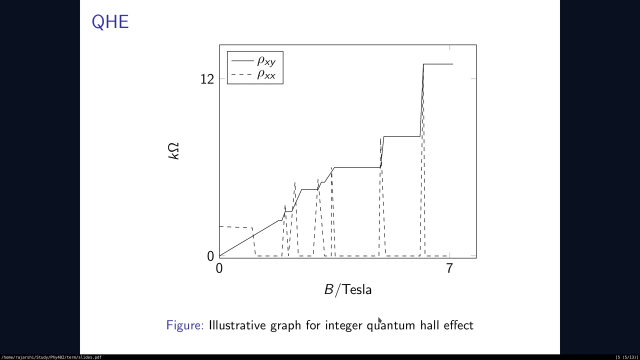 the relaxation time tau. So when we assume the steady state for this equation from the Drude's model, we obtain values of rho x x and rho x y, And indeed rho x- y is seen to be proportional to B, as we expected To experience. to observe quantum effects we have to go to extremely low temperatures. 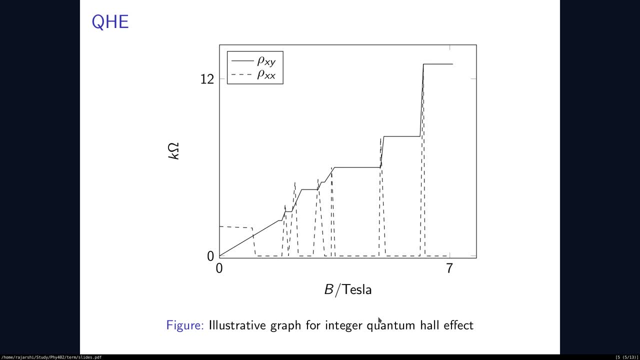 and we have to vary the magnetic field to very large values, because even values of 1 tesla and 2 tesla are actually very large. So once we do this for large magnetic field, we see that rho xy has forms, plateaus, that 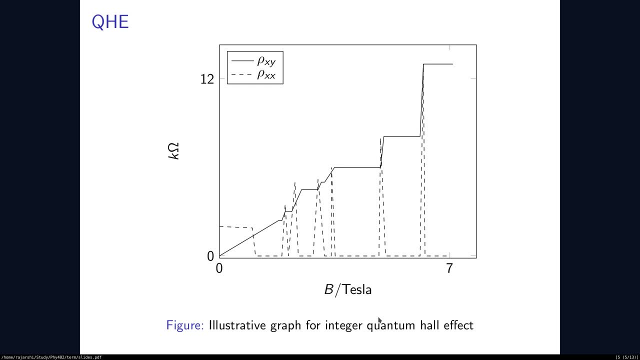 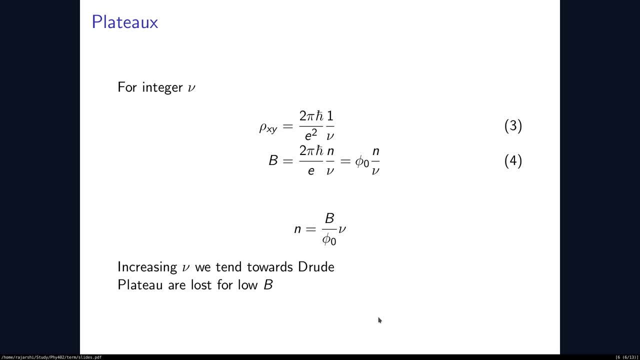 is for a certain interval of a magnetic field, rho xy gets fixed and rho xx goes to 0.. The features of this graph is captured by these equations. So rho xy is inversely proportional to an integer, and so is the magnetic field. In this formula, if we increase mu, 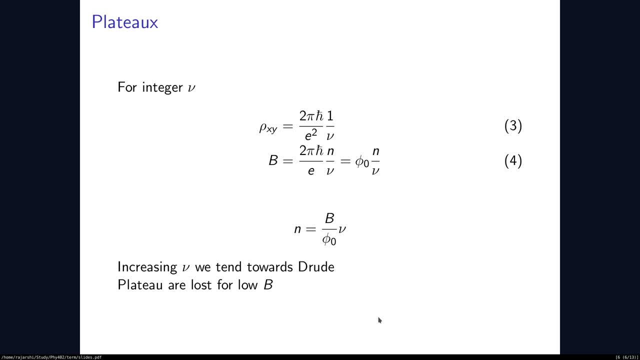 Then we get b and rho to be continuous, because nu is very small. So rho and b, the differences in rho and b, becomes very small and rho and b become continuous and they are proportional. So that is what is proposed by the. that is what is predicted by the Drude's model. 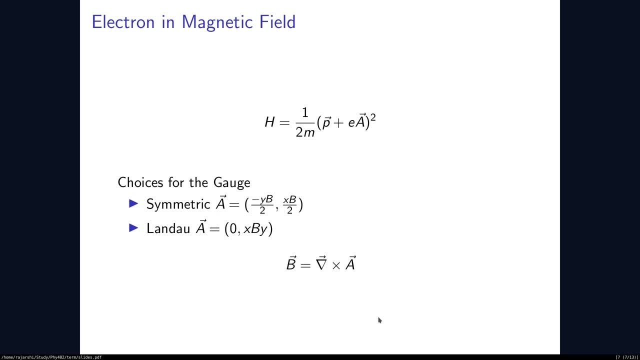 To understand this phenomena, In this quantum phenomena, we have to understand the quantum mechanics of the electron in a magnetic field. For doing so, we have to deal with the Hamiltonian, in which the vector potential A is involved. and as the story goes, with the vector potential A, there are several choices for A, two of 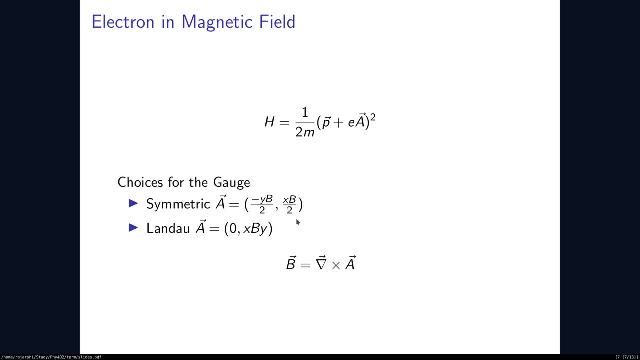 them are called. two of them are shown here. one is called the symmetric gauge and one is called the Landau Gauge. The use of the Landau Gauge is very interesting that in the Landau gauge we can calculate the degeneracy of the levels. 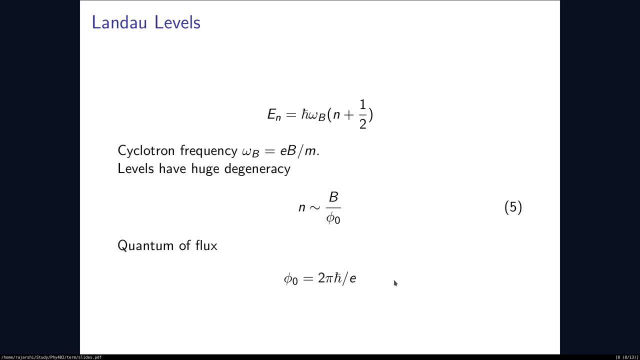 very easily. So once we do that, we find that the Landau levels are equispaced, that is, the energy levels are equispaced and they are given by this formula: h cross omega b. So the spacing between the energy levels is h cross omega b and each level has a degeneracy. 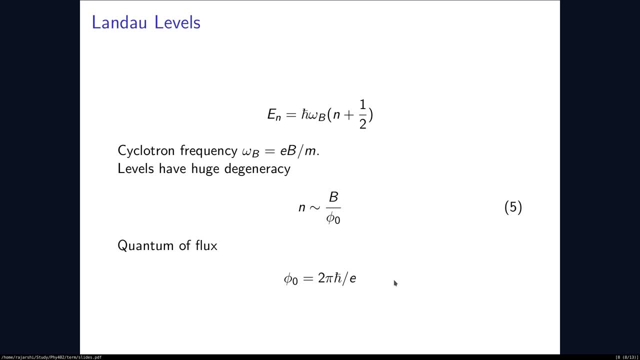 So the number of electrons per unit area is going to be b by phi0, where phi0 is a quantum of flux to be given by this lowest equation. So what happens is there are several states and when exactly mu of them are fix, we find something interesting. We find when that over. 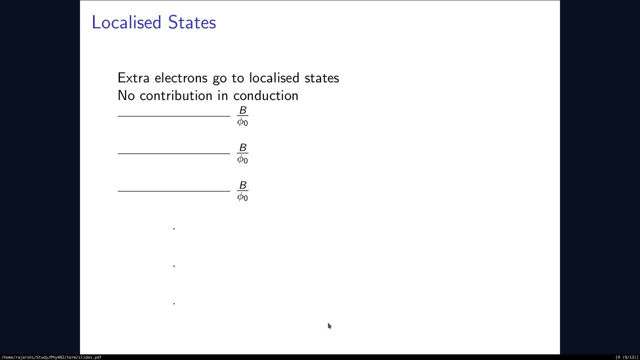 here, when exactly mu of the energy levels are filled, are completely filled. then we find this: the predictions by the experiment. So rho x, y is fixed and b is fixed, To understand what happens for the magnetic field which is not given, which is which is not an integral. 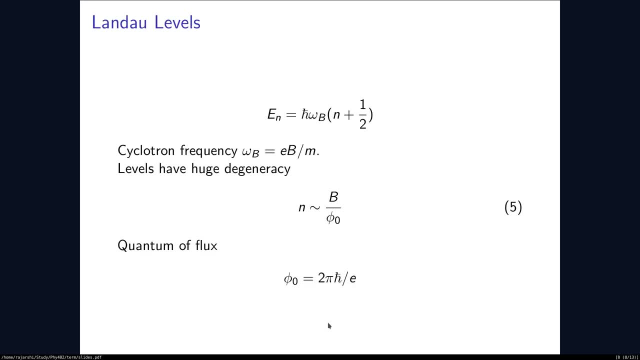 multiple of b by phi naught. we have to consider the potential created by disorder in the crystal, that is, the impurities and defects which are there in the crystal, and these have to be significantly lower than h cross, omega b, which is the energy scale of the Landau levels, and 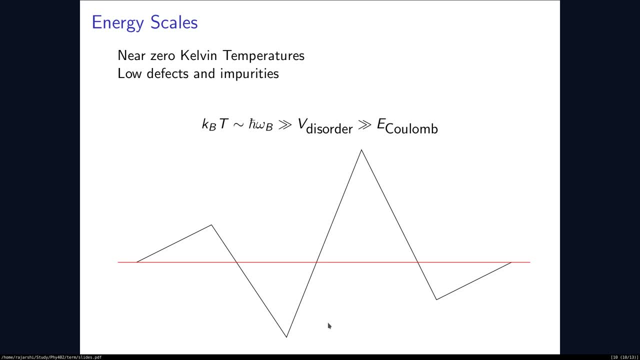 the energy scale of the Landau levels have to be comparable to the temperature k, B, T, right. So what happens is that the V disorder forms crests and troughs. So V disorder forms energy states which are very localized. So once an electron is in a trough it is very difficult. 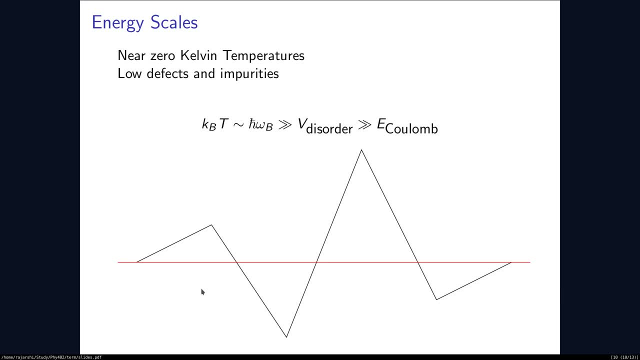 for it to get outside, because it has to tunnel through and because of this reason the energy states created by the V disorder do not contribute to the conduction. So over here we say that the disorder is larger than the Coulombic repulsions. So what? 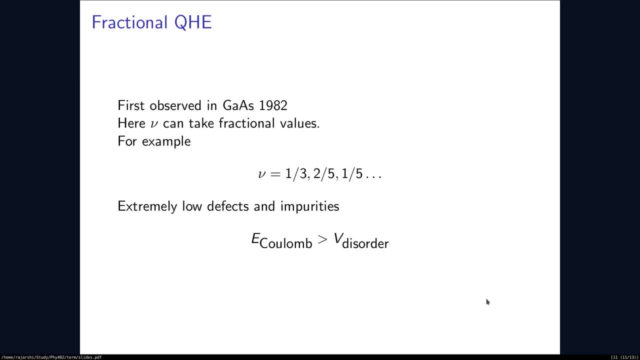 happens if you take a very pure crystal. So in this case we see the fractional quantum Hall effect. So in this you can take certain fractional values, So nu equal to 1 by 3,, 2 by 5, 1 by 5, so these are observed. So to explain this we have to consider the Coulombic. 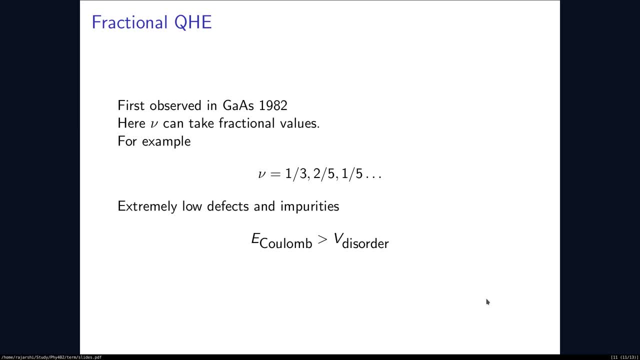 repulsions in the Hamiltonian. The further scope which we gain by understanding the integer quantum Hall effects is first to study the fractional quantum Hall effects, and for that we have to understand log-lean states There are. instead of that, you can also look at the conduction on the edges, because 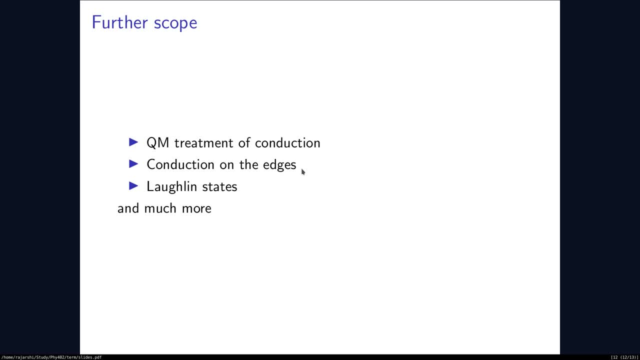 in the edges there is some charge accumulation and that is a one dimensional problem that also we can explore, and there are many more such topics. For now, this is all. Thank you very much.